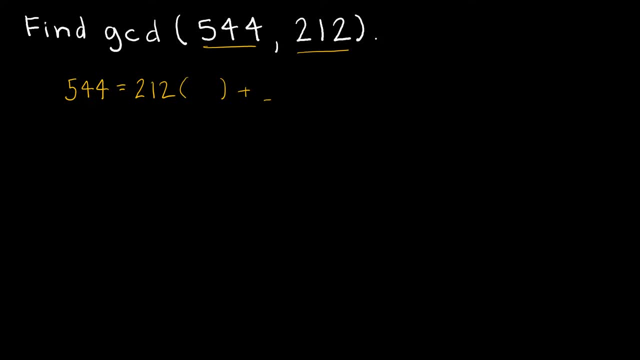 212 times something plus something. So this process should look familiar to you because we've done it before. So if I were doing this, I would find that 212 times 2 with a remainder of 120 is the same as 544.. So now let's continue this process. What this tells me? 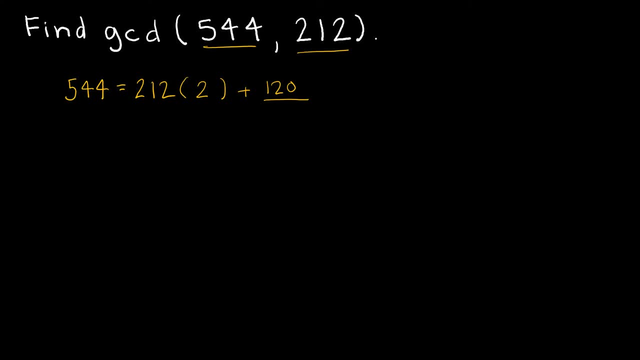 is that the GCD of 544 and 212 is the same as the GCD of 212 and 120.. 212 and 120.. And notice the 212 just carried over. So now we're going to start with 212.. 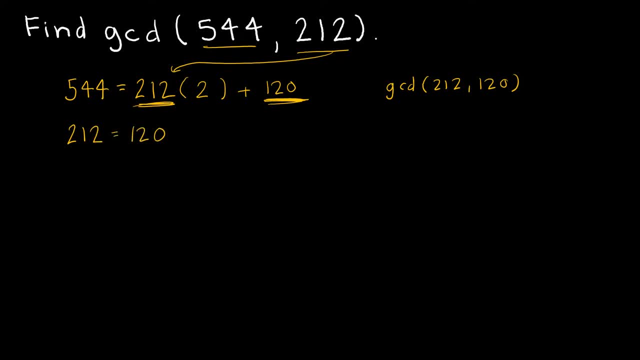 And say 212 is equal to 120 times some number plus some number, And in this case 212 would be equal to 120 times 1 plus 92, which means this GCD is the same as the GCD of 120 and 92. So now let's find the GCD of 120 and 92.. 120 equals 92 times. 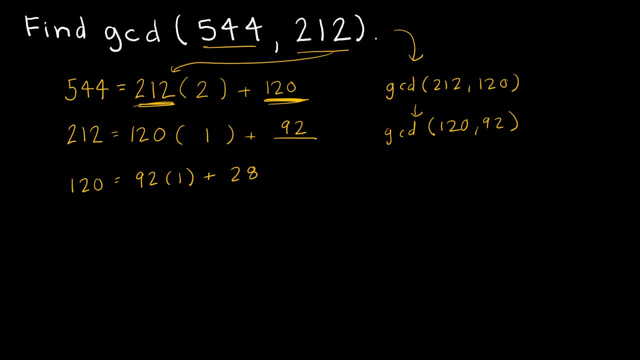 1. plus 28. so now i'm trying to find the GCD of 92 and 28. So I say 92 is equal to 28 times 3. Plus eight. So now I'm trying to find the GCD of 28 and 8. Then I'm going. 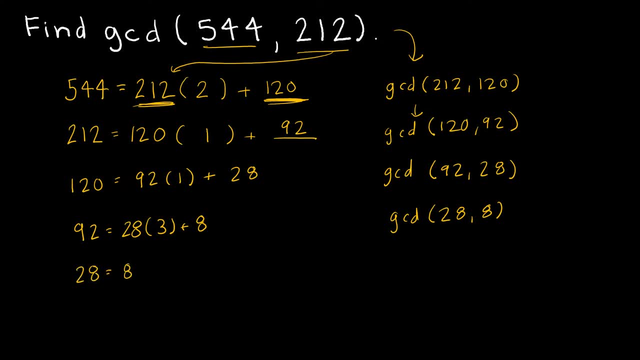 to say, 28 is equal to eight times 3 plus 4.. So now I want the GCD of 8 and 4.. Now 8 is equal to 4 times 2 plus 0. So once I get to a remainder of 0, that's when I'm done. So don't get confused The other time that we did this 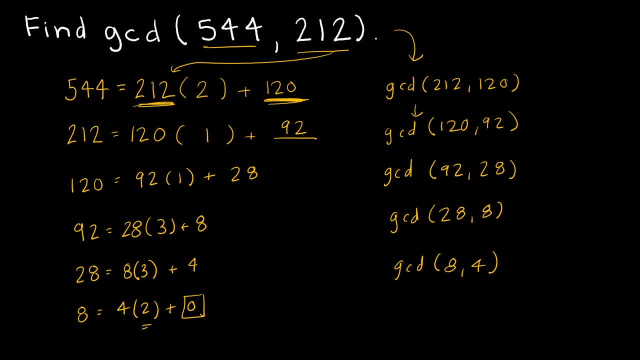 when I said your quotient had to be 0,. once I get to a remainder of 0,, then I know that I'm done. Now, what is the GCD? The GCD is the last remainder, which is whatever number you're carrying down. 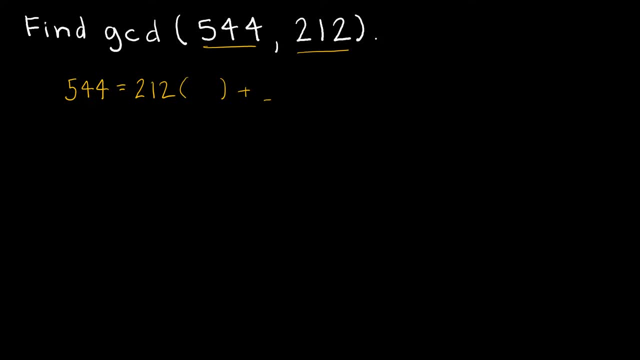 212 times something plus something. so this process should look familiar to you because we've done it before. So if I were doing this, I would find that 212 times 2 with a remainder of 120 is the same as 544.. So now let's continue this process. What this tells me? 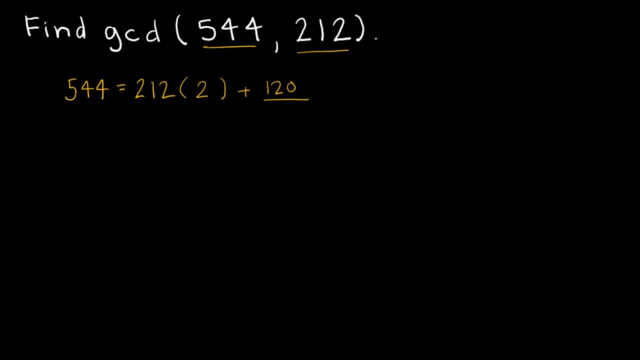 is that the GCD of 544 and 212 is the same as the GCD of 212 and 120.. 212 and 120- and notice the 212 just carried over. So now we're going to start with 212. And say 212 is equal to 120 times some number plus some number. and in this case 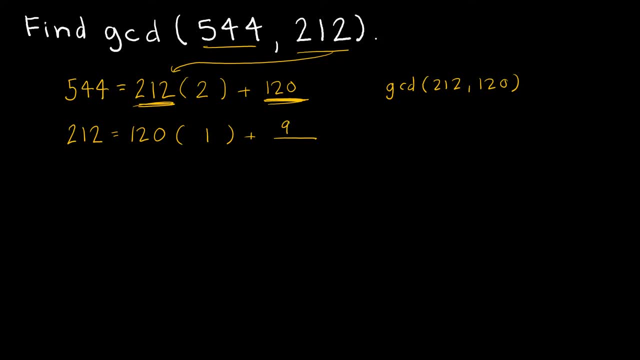 212 would be equal to 120 times 1 plus 92, which means this GCD is the same as the GCD of 120 and 92. So now let's find the GCD of 120 and 92.. 120 equals 92 times. 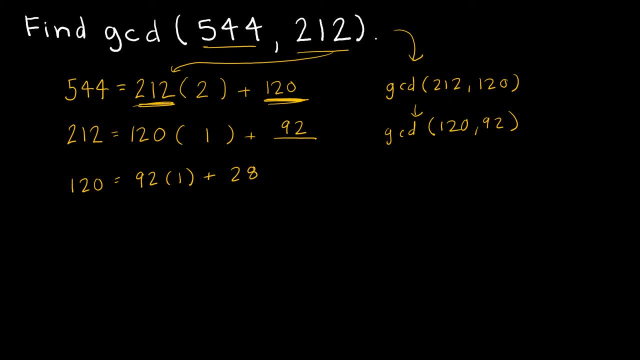 1. 8 plus 1 plus 28. so now I'm trying to find the GCD of 92 and 28.. So I say 92 is equal to 28 times 3 plus 8.. So now I'm trying to find the GCD of 28 and 8. then I'm going to say 28 is equal. 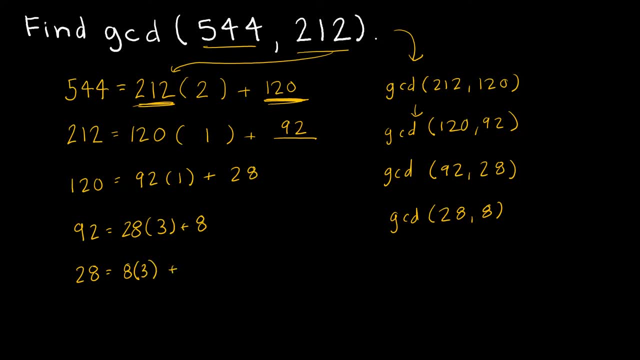 to 8 times 3 plus 4.. So now I want the GCD of 8 and 4.. Now 8 is equal to 4 times 2 plus 0. So once I get to a remainder of 0, that's when I'm done. So don't get confused The other time that we did this 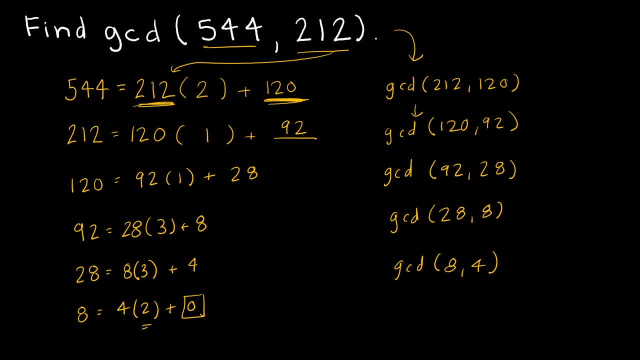 when I said your quotient had to be 0,. once I get to a remainder of 0,, then I know that I'm done. Now, what is the GCD? The GCD is the last remainder, which is whatever number you're carrying down. 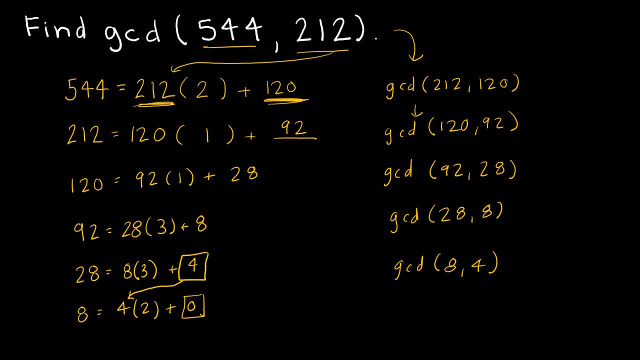 whatever the last quotient would be. So in this case, then, the GCD would be 4.. So this GCD is 4 because it's the same as the GCD of all of the other representations that I had. That is how we. 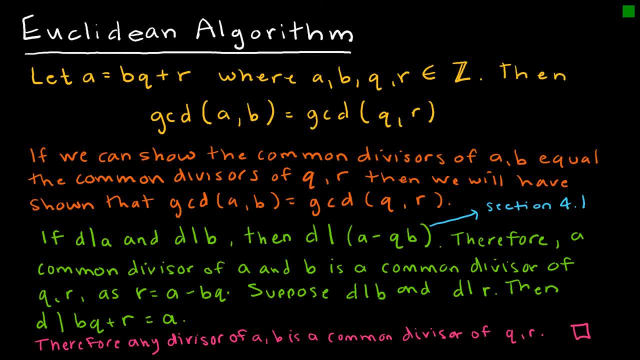 use the Euclidean algorithm. So now let's take a look at the actual algorithm, or what the algorithm says. It says: let A equal BQ plus R. Again, we're used to that format. We're saying it's some number times a quotient plus a remainder, where A, B, Q and R are all integers, Then the GCD the greatest. 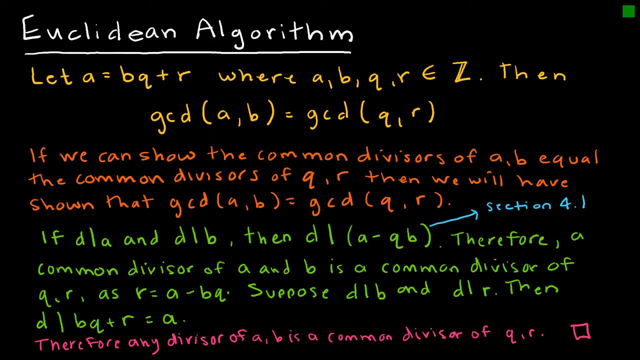 common divisor of A and B Is equal to the greatest common divisor of Q and R, which is, of course, the quotient and the remainder. So that is what the Euclidean algorithm says and that's what we put into play just a few moments. 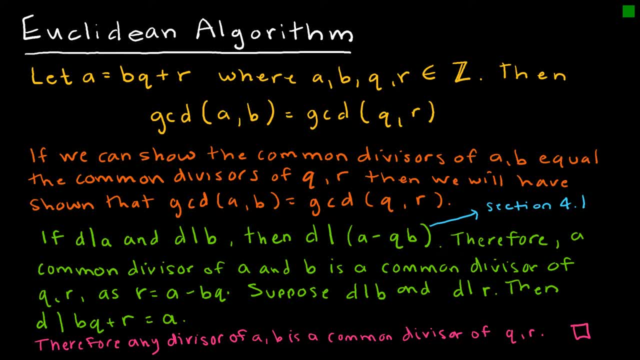 ago. But why does this work? So again, if I want to prove this, then I want to show that the common divisors of A and B are equal to the common divisors of Q and R, because if all of those common divisors are equal, then we know that the greatest common divisor of A and B is the greatest. 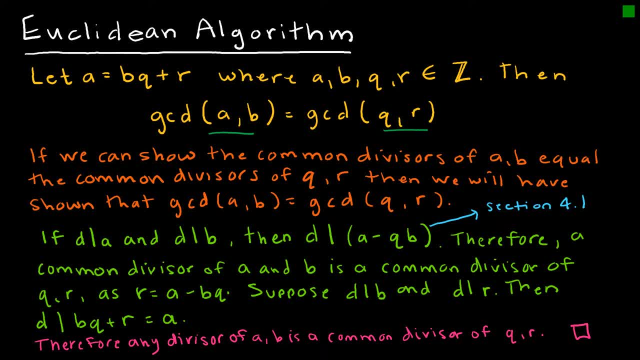 common divisor of each is equal, because all of the divisors are equal. So then, to go about proving it, I'm saying: if D divides A and D divides B, so D is a divisor for both A and B. then D also divides the quantity of A minus QB. 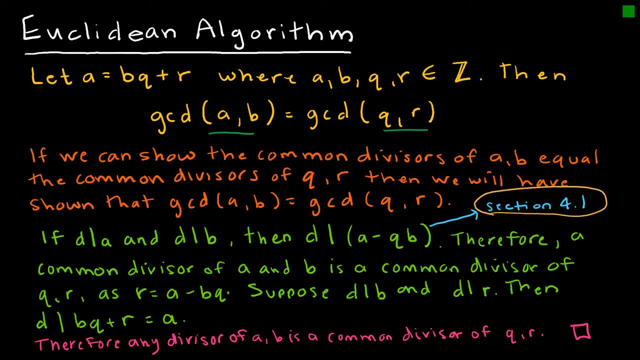 Now, I didn't provide a proof for that, but in section 4.1, we did go through that. you know, if D divides A and D divides B, then D divides A plus B, and I believe we also went through the proof where we said: 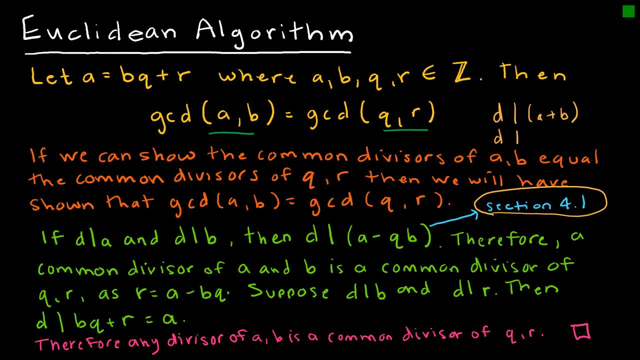 if D divides A and D divides B, then D divides A times B, and so it follows from there. So therefore, a common divisor of A and B is a common divisor of Q and R, because again we're saying D goes into this, which means and R. 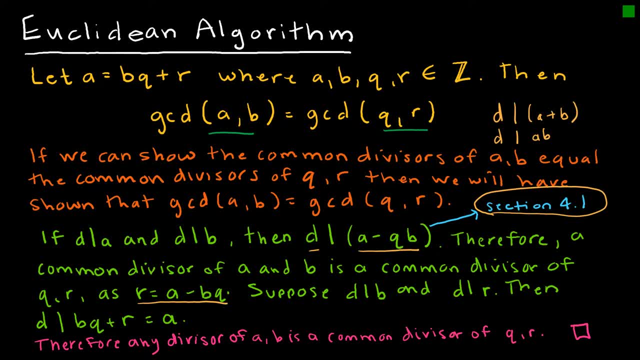 is obviously A minus BQ. So then we suppose: so this is sort of an if and only if statement, and remember if and only ifs. we have to go in each direction. So then we suppose that D divides B and D divides R, then we can say that D divides BQ plus R. 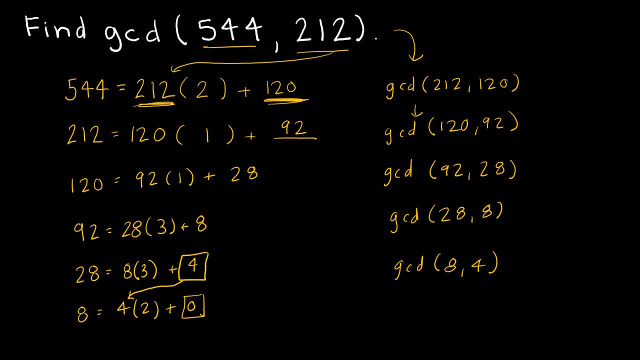 whatever the last quotient would be. So in this case, then, the GCD would be 4.. So this GCD is 4 because it's the same as the GCD of all of the other representations that I had. That is how we. 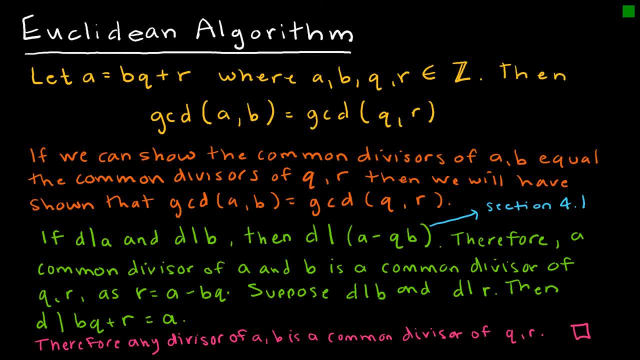 use the Euclidean algorithm. So now let's take a look at the actual algorithm, or what the algorithm says. It says: let A equal BQ plus R. Again, we're used to that format. We're saying it's some number times a quotient plus a remainder, where A, B, Q and R are all integers, Then the GCD the greatest. 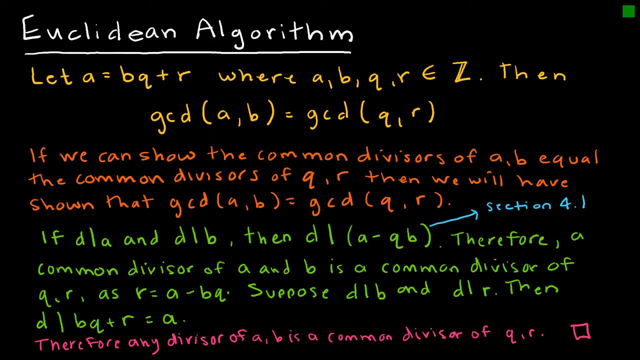 common divisor of A and B Is equal to the greatest common divisor of Q and R, which is, of course, the quotient and the remainder. So that is what the Euclidean algorithm says and that's what we put into play just a few moments. 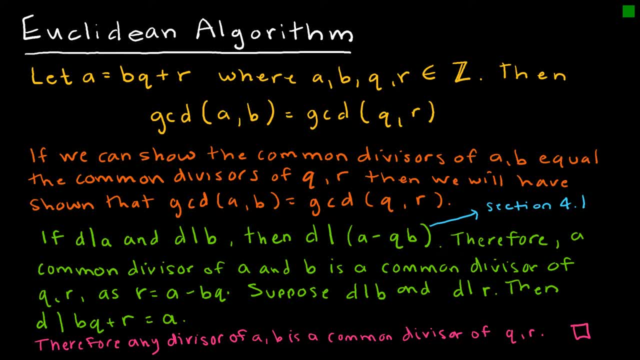 ago. But why does this work? So again, if I want to prove this, then I want to show that the common divisors of A and B are equal to the common divisors of Q and R, because if all of those common divisors are equal, then we know that the greatest common divisor of A and B is the greatest. 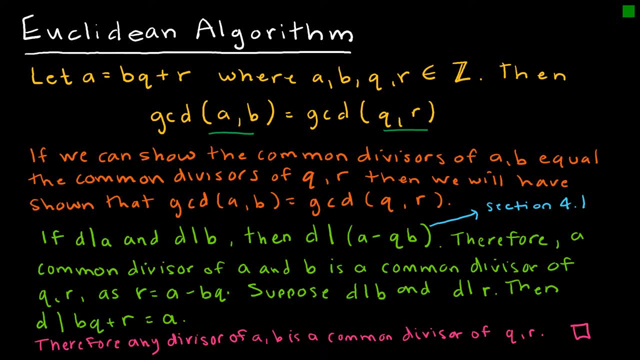 common divisor of Q B divided by R. So an interesting thing to build here is that if the corresponding divisors- those are opportunities to ask is what the true nature of GCDs And yellow are to be trove-divided as effective and yellow are to clear the meaning of display. Similarly, if D is 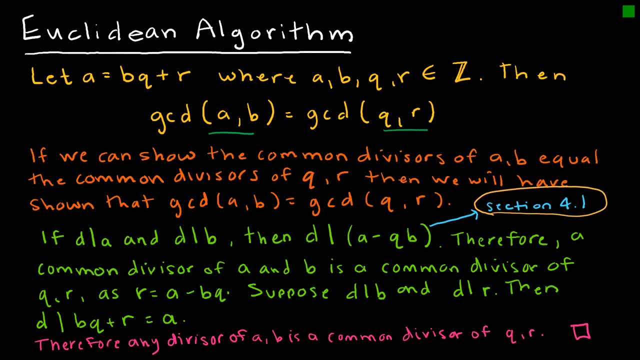 not a divisor for R, then can it be a divisor for both A and B? Or it might be that D divides A and D divides B. then we know this, as D divided for both C and D are equal. So that's the proof. 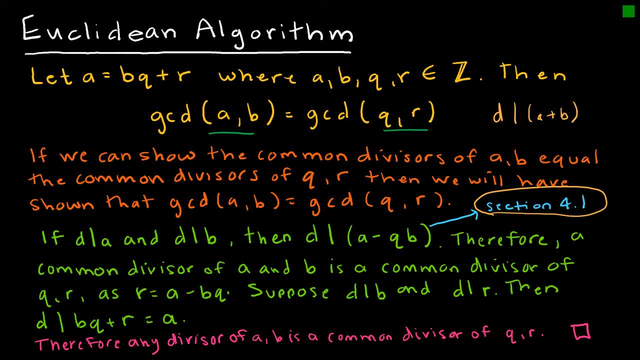 This is proof: D divides A plus B, and I believe we also went through the proof where we said if D divides A and D divides B, then D divides A times B, and so it follows from there. So therefore, a common divisor of A and B is a common divisor of Q and R, because again we're saying D goes. 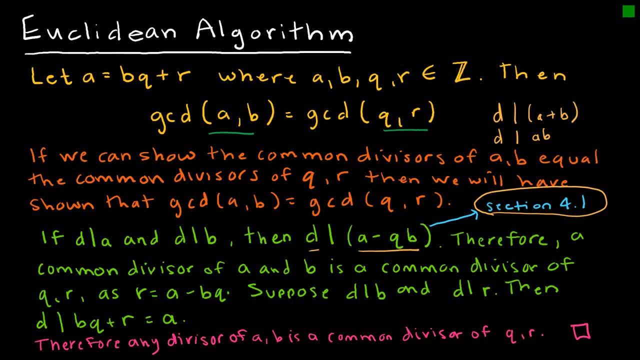 into this, which means: and R is obviously A minus BQ. So then we suppose: so this is sort of an if and only if statement, and remember, if and only ifs. we have to go in each direction. So then we suppose that D divides B and D divides R, then we can say that D divides.